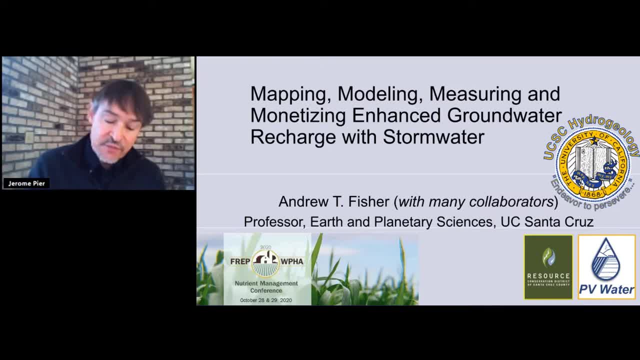 He also serves as the US Santa Cruz Director for UC Water, a co-PI for the Center for Dark Energy Biosphere Investigations and the founder of the Recharge Initiative, which is an organization that you could go find online. So the Recharge Initiative is a focused effort to protect, enhance and improve the availability and reliability of groundwater resources. 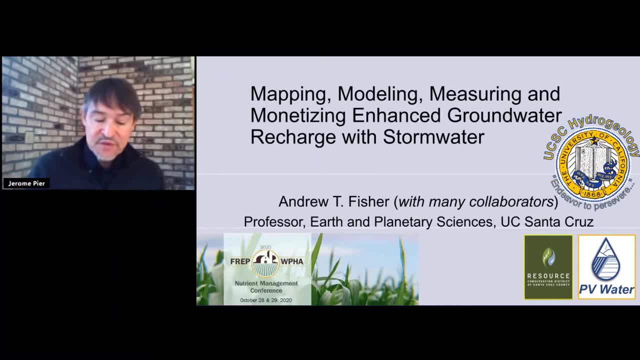 Dr Fisher has authored or co-authored over 200 articles, books, chapters, reports and other documents and supervises. He has supervised 24 grad students and more than 50 undergraduate researchers and he does a whole lot of stuff. so we're really honored to have him. and take it away, Andy. 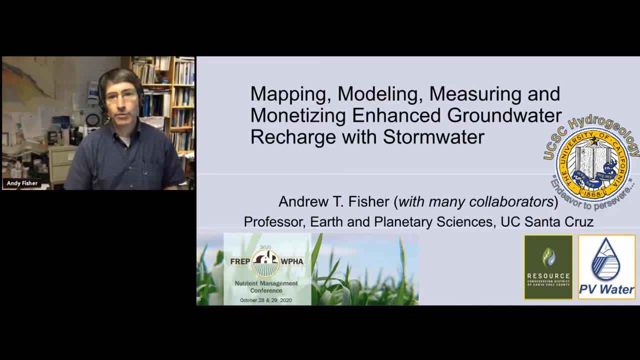 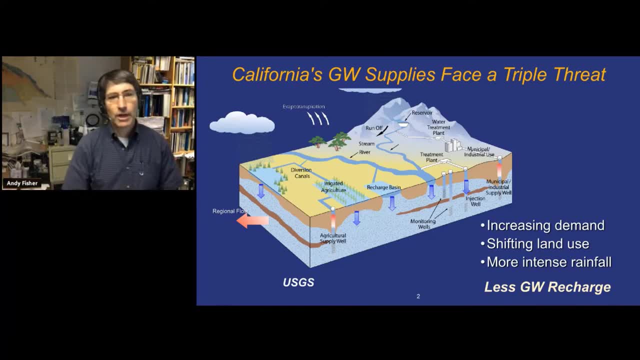 Thank you very much. It's really been fun to be here and I appreciate the opportunity to spend a few minutes with you. So in general in California there are really three major threats to water supply. Of course, increasing demand is one of the big ones. But two others that folks may not think about as much are shifting land use and the increase in intensity of rainfall- Not a change in the total rain, but the fact that more rain is falling during a smaller number of more intense storms. Both of these last two factors tend to make more water run off the landscape, and that results in less groundwater recharge. 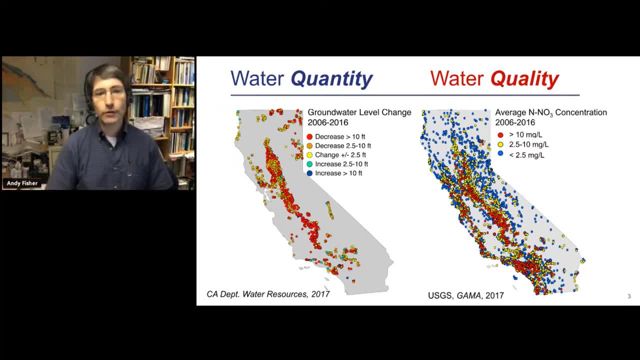 Now the challenges to California go from quantity to quality. This diagram shows, on the left-hand side, Groundwater level changes over a 10-year period, the second half of which includes the recent drought, and those circles that are in red and orange indicate water level declines of two and a half feet or more. 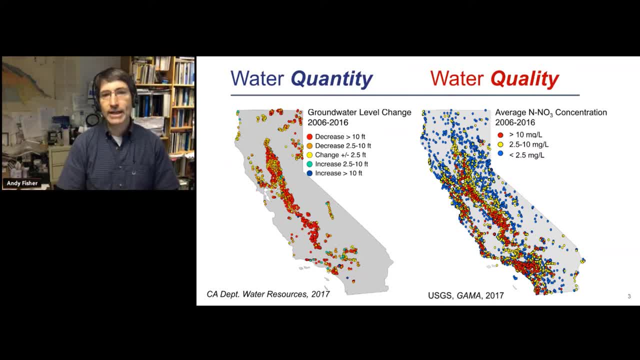 On the right we see measurements of water quality highlighting nitrate and nitrogen in groundwater, and the dots that are in red are above the drinking water standard and even those that are in yellow are pretty high, and many of those actually that are blue are above background levels. 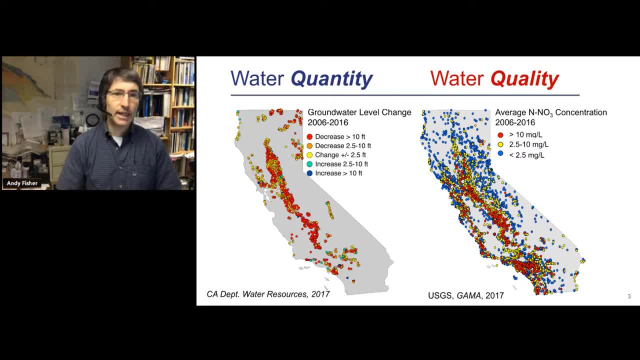 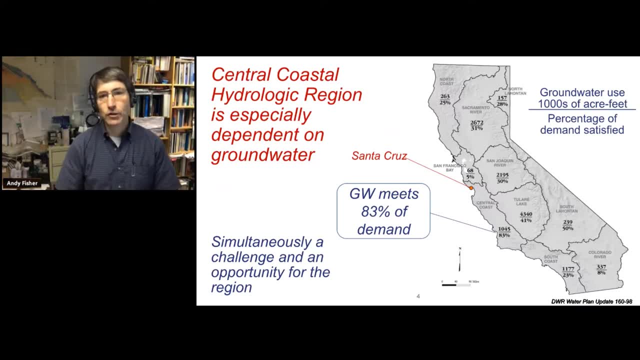 Well, what you can see is there is a Correlation between the decline in water quantity and the decline in water quality. Here on the central coast, we're especially dependent on groundwater. We don't use more groundwater than other parts of the state, but we use a larger percentage of groundwater in order to satisfy our freshwater demand. 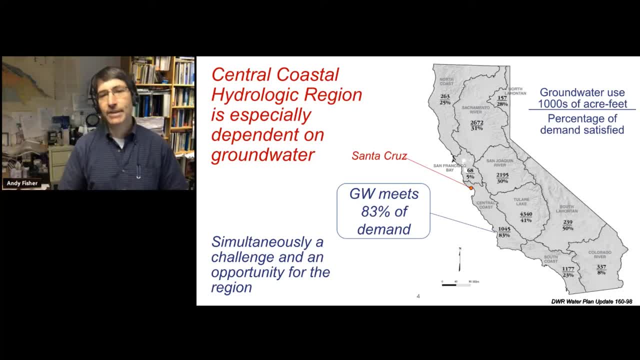 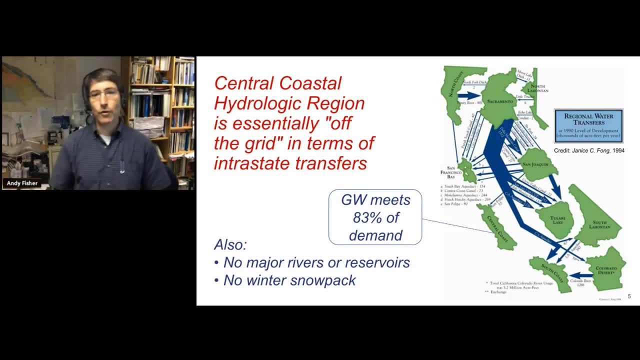 And that's a big challenge for us, but it also provides potential opportunities because that dependence is so strong, And part of the reason the dependence is so strong Is because we have no choice. We're essentially off the grid in terms of this massive interest state transfer system and also we have no major rivers like the kind you see in other parts of California that provide these excess flows that can be transferred around, and we have no winter snowpack of significance. 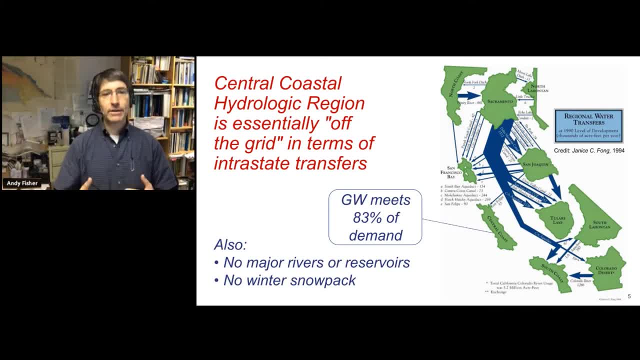 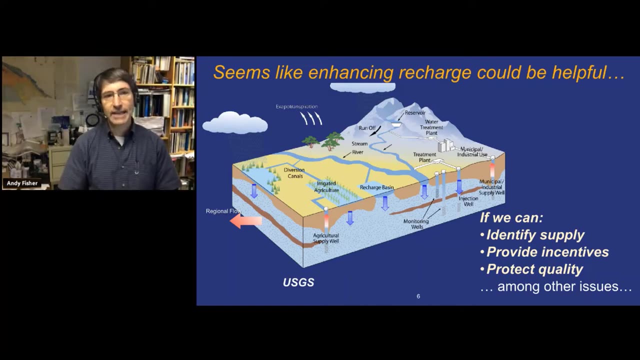 So every year we're dependent on what happened that year and the previous year and maybe a couple years before, but we really are watching That precipitation each year. So it sounds like enhancing recharge could be helpful, but there are a variety of technical and economic and policy challenges that are associated with that. 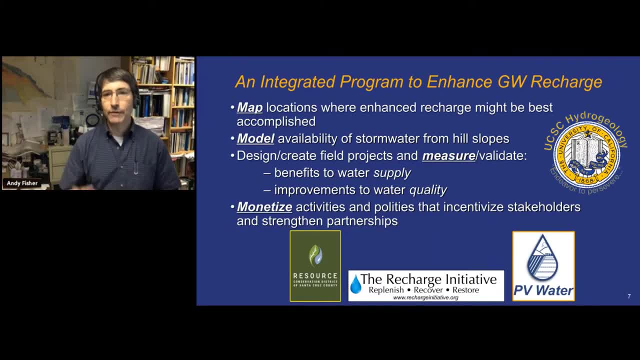 And I'm going to just give you a whirlwind overview of a couple of those and talk about some of the things that we're collaborating on in the Pajaro Valley. So the recharge initiative is really trying to do a number of things. We're trying to map and identify locations where recharge might be a conflict. 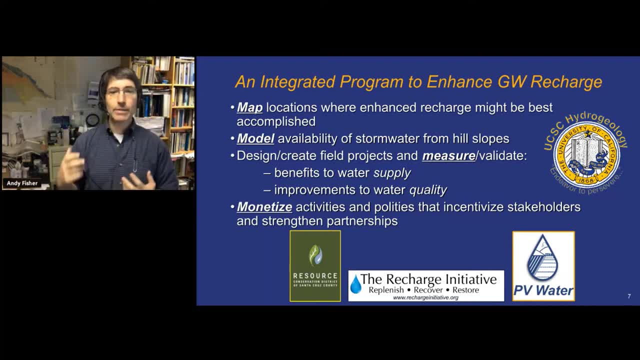 We want to model the availability of water, help to actually build projects where we can measure benefits, both the supply and quality, and then we've been engaged in this incentive program that I'll tell you about in in a moment. So first I want to just discuss managed recharge a little more broadly. 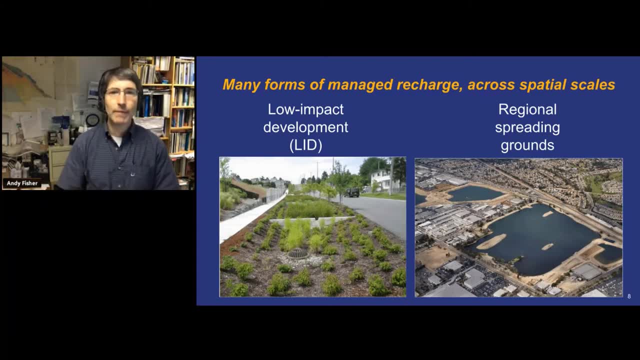 There's sort of two extreme end members that many people may be familiar with: Low impact development. This is small projects that are typically located close to the source, where runoff is generated, and then large Regional spreading grounds where waters piped in, often from great distance or maybe from a large recycling plant. 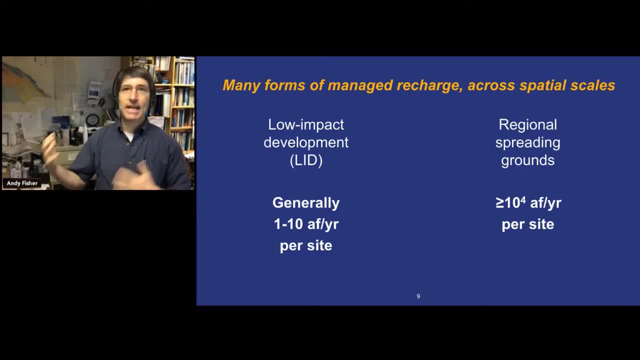 And these really differ in scale. LID tends to generate an acre foot or two per year. Regional spreading ground projects can be huge, like in Orange County or Santa Clara Valley, and can generate over 100,000 acre feet per year per site. 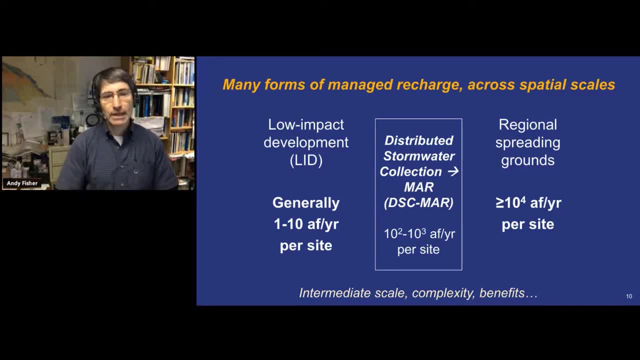 We've been kind of focusing at an intermediate scale where we think there's a lot of opportunity, potentially at relatively low cost cost and with only modest engineering effort. And this is what we call distributed stormwater collection, leading to managed aquifer recharge. 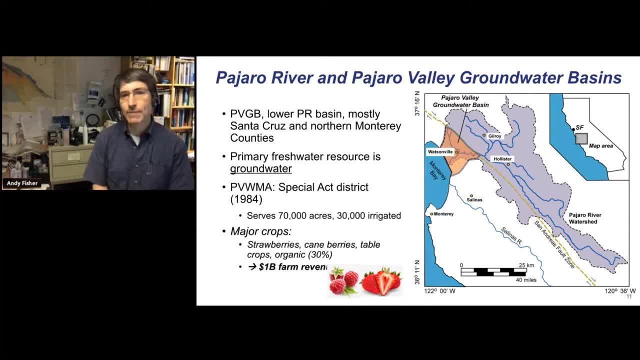 So Brian's told you about Pajaro Valley. I'm not going to spend much time on it, but I'll just note that it really is the value of the ag that's providing much of the incentive to develop programs to help to balance that aquifer. 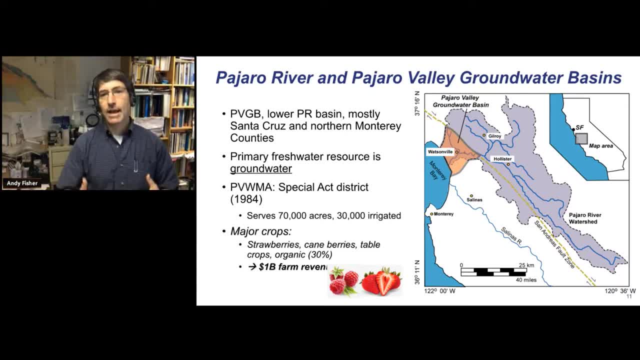 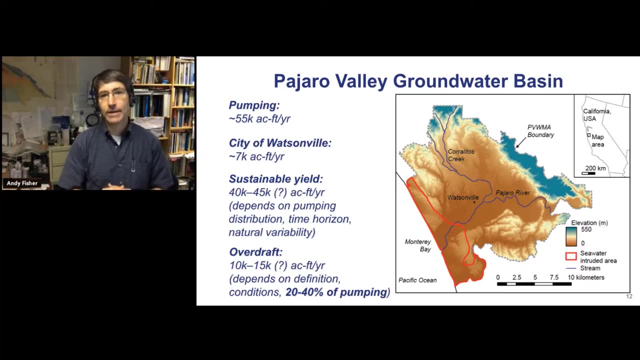 And in that area, which is a very small region, it has quite a large economic base, Not just the crop production but all the ancillary work that goes on, and then all the other social and economic activity that's created by all of that activity. 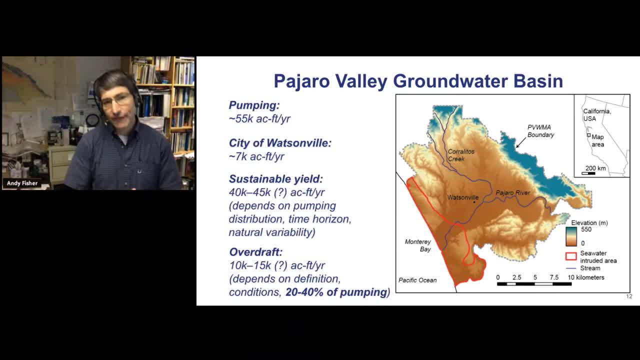 And, as Brian mentioned, the overdraft in Pajaro Valley. it varies year by year. it depends on the rain, it depends on the pumping, But what you're looking at is something on the order of 20 to 40 percent of annual. 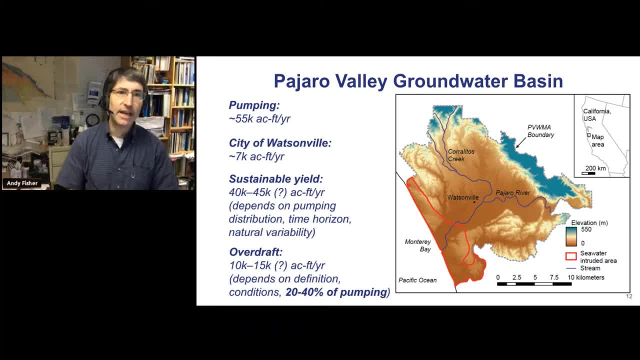 pumping, at least as of about 5 to 10 years ago. As Brian noted, things are starting to head in a very good direction, but there still is a deficit and the goal of the basin management plan is really to balance the basin by finding 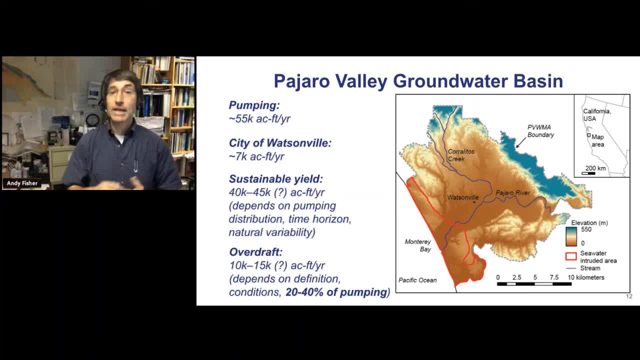 a combination of about 12,000 acre feet of increased supply and reduced demand And of course, it's that imbalance which is leading to the seawater intrusion along the coastal area. So here's one example of a project. This is a project that we've been helping with. 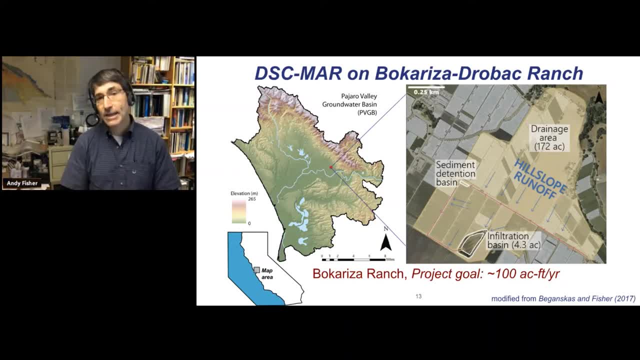 And this is on Boca Riza Ranch sort of towards the back, the eastern side of the basin And in this area, runoff from around 170 acres of agriculturally developed landscape, is directed towards a series of ditches and culverts through a small sediment detention basin. 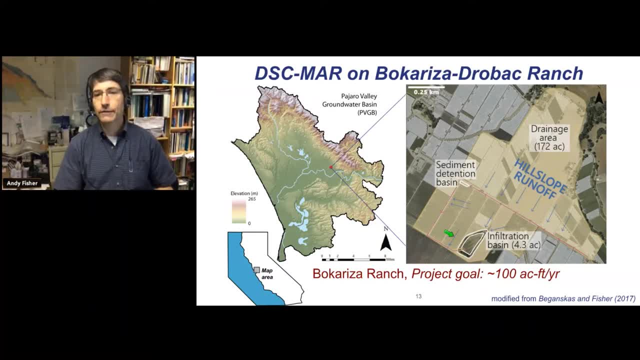 And then eventually into this infiltration basin located here. The concept of the project is to calculate. The project is to capture some of the big runoff events that occur during intense rainstorms and then direct some of that water to a location where it can infiltrate relatively rapidly. 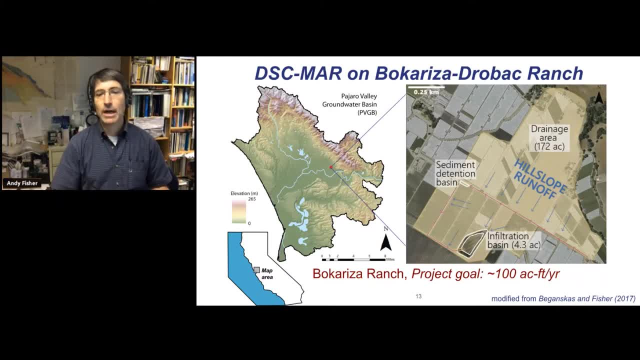 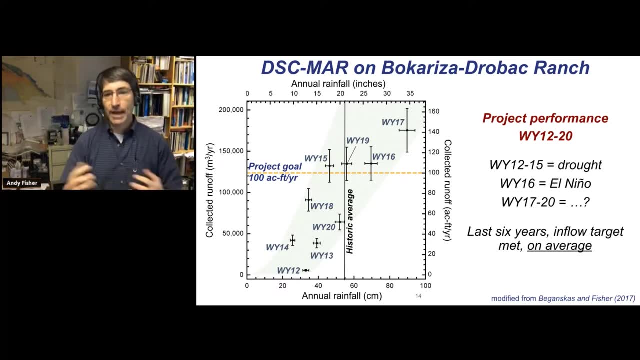 And the general goal is to get about 100 acre feet per year during an average water year. Here's a summary of nine years in which we've been monitoring at the site and helping to try to improve performance. On the x-axis we see rainfall centimeters and inches. 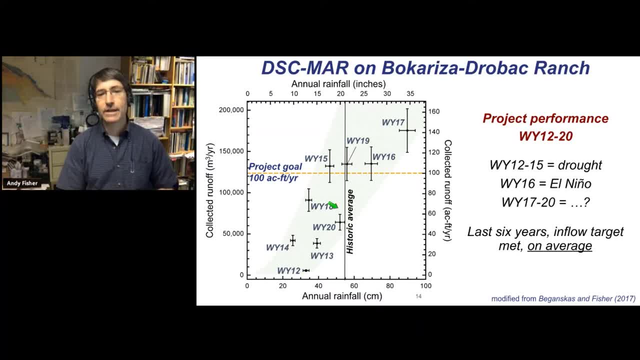 And then the y-axis is runoff. That was collected acre feet here and cubic meters on the left. When we started work it was during the drought And it really looked like we weren't going to get much benefit out of this project. But what you see is that for the last six years, if you average these flows together, 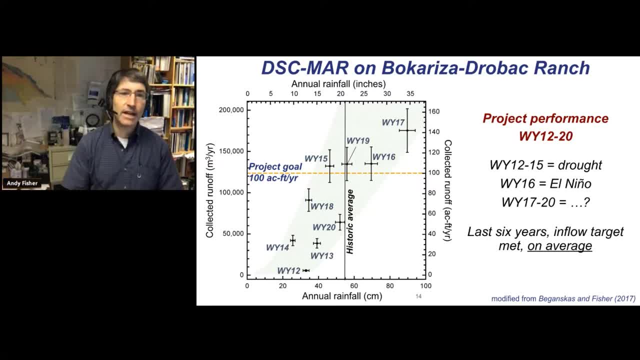 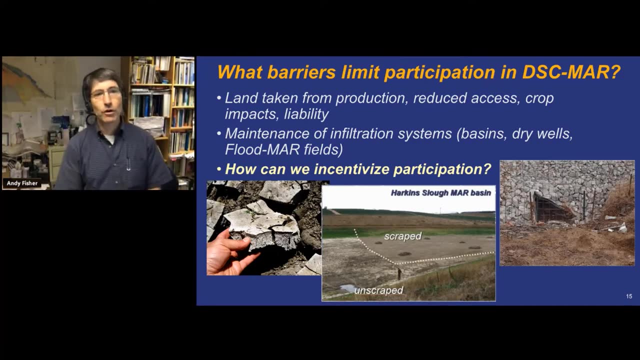 we hit the goal for the project of getting about 100 acre feet of additional water into the ground, So this seems to be viable and it seems to be meeting its objectives in terms of water supply. Next slide. But a challenge is that projects like this do require operation and maintenance, and 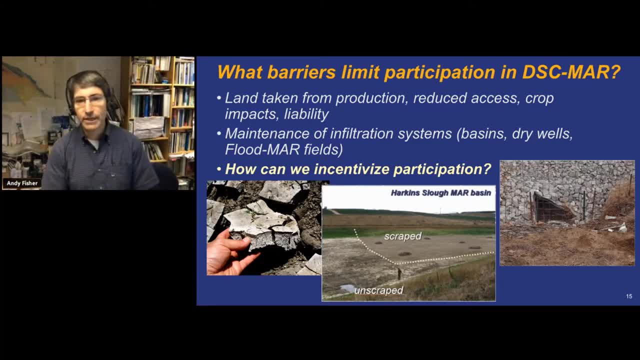 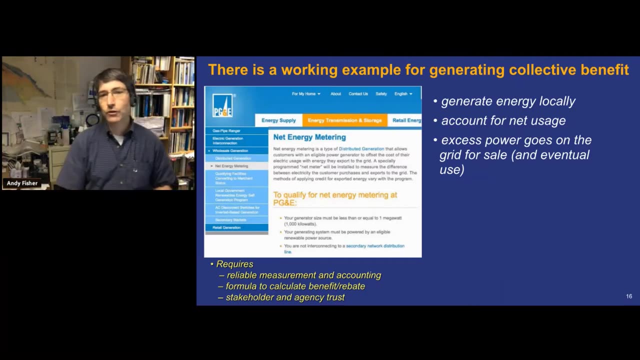 they occupy land that could be agriculturally productive. So it's important, if projects like this are going to be done, that we provide some kind of an incentive which can offset these really real costs that the stakeholders who are involved are seeing, And there's a model for this that we look to. 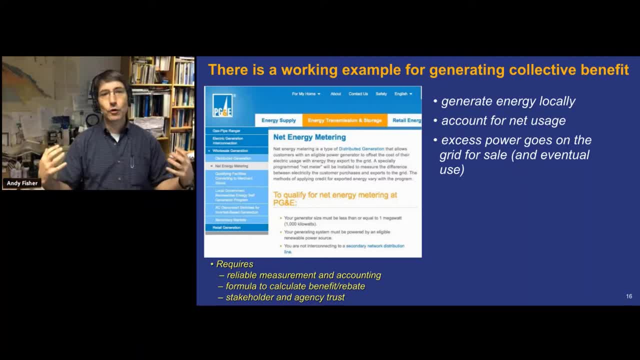 This is net energy metering. This was the idea that you could put solar panels on your house, generate power and if there's more energy than you need, then some of that excess can be put back on the grid and you get a credit. 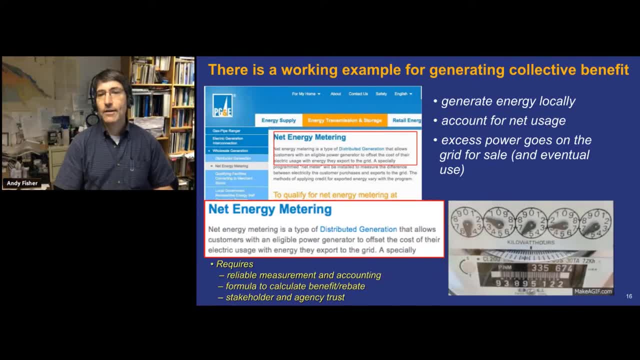 So that idea is relatively straightforward and it has been successful in California in helping run their meters backwards by generating excess power. So what does this really require? Well, you need to be able to measure the benefit. You need a formula for calculating what the rebate or payment is going to be. 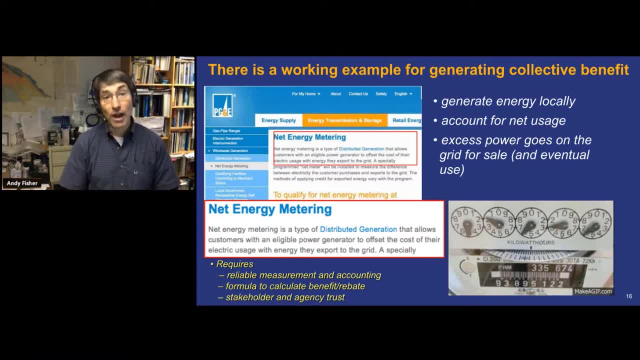 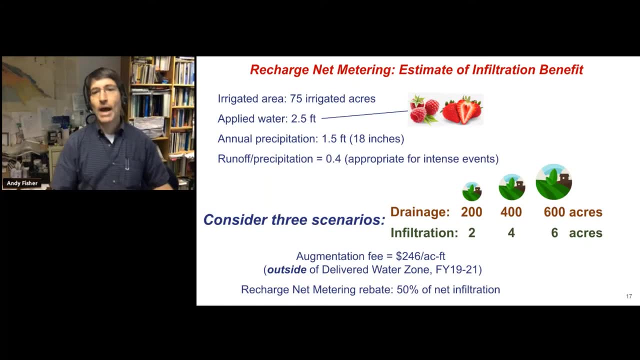 And, of course, you need to establish relationships based on trust: Those who are supporting the project and those who are participating in the project. So how would this look? Well, imagine you've got 75 acres growing delicious red berries, maybe two and a half. 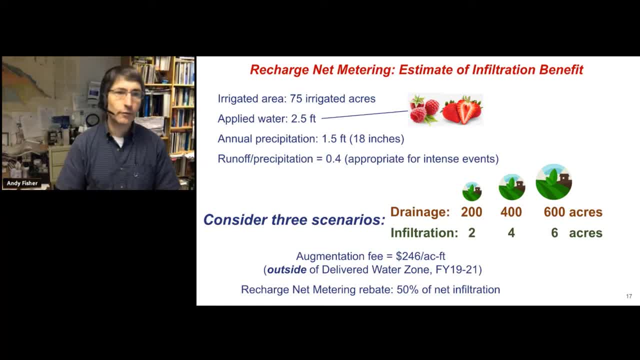 feet of water in an area where there's 18 inches of rain a year in the southern part of the Pajaro Valley. We assume a certain runoff coefficient based on measurements we've made in the field. Now imagine three scenarios: Drainage areas of 200,, 400, or 600 acres. 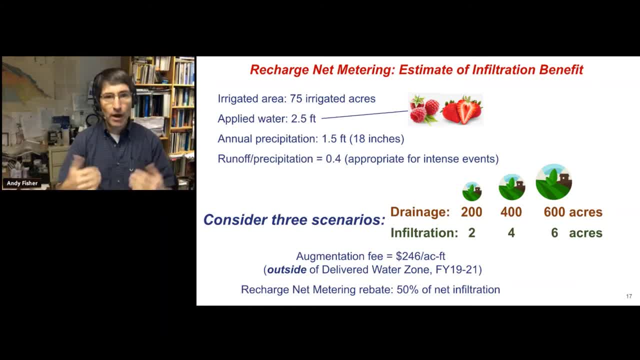 The larger the drainage area, the higher the cost. The more of this excess runoff could potentially be routed towards an infiltration basin. And let's just assume, somewhat arbitrarily, that 1% of that drainage area is now allocated to infiltration In much of the Pajaro Valley. the pumping augmentation fee is about $250 an acre foot. 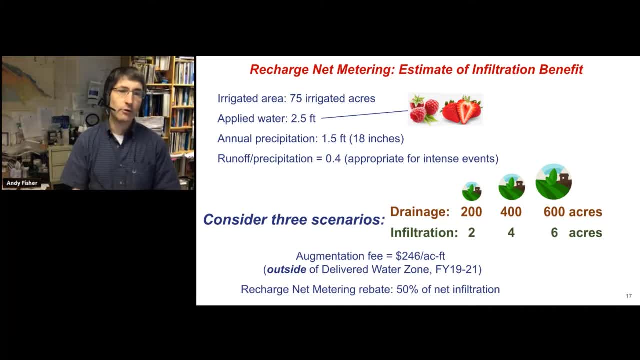 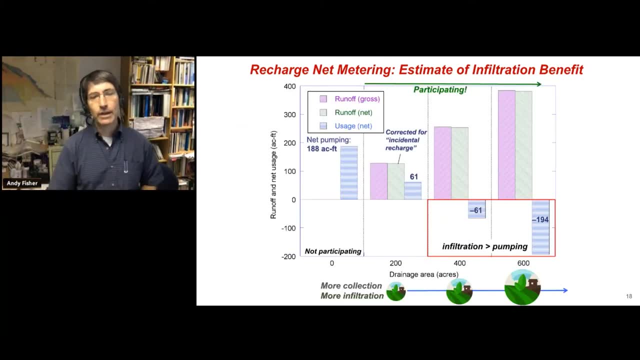 and we'll assume here a 50% rebate. So you get 100 acre feet in the ground. you get a payment equivalent to the pumping cost for 50 acre feet. So here's how that would pencil out. Imagine on the left we have a non-participating grower, pumps about 190 acre feet, pays for 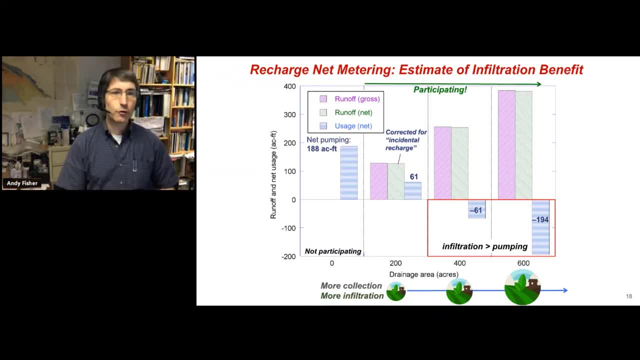 that water. Now you have three other growers who participate with drainage areas of 200,, 400, or 600 acres. We do a calculation to correct for the incidental infiltration that would have occurred anyway. We don't account for that as a benefit. 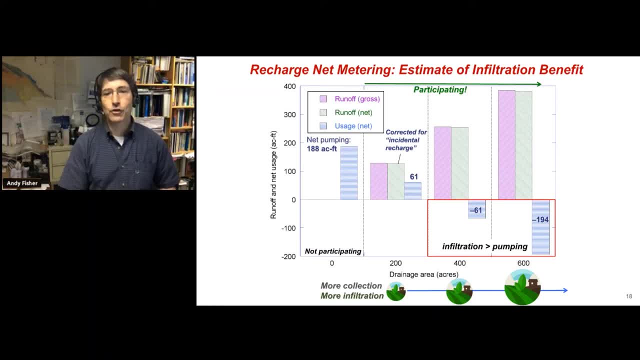 And then what's left is this infiltration benefit, And for 200 acres of drainage, you get about 60 acres of drainage. So that's a benefit. And then what's left is this infiltration benefit, And for 200 acres of drainage, you get about 60 acres of drainage. 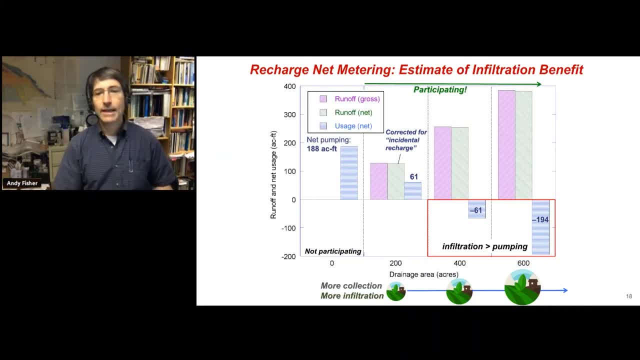 So that's a benefit. So the net pumping is reduced. In the case of 400 to 600 acres of drainage, you actually have so much infiltration that the net pumping is negative. In other words, more water is being put in the ground than is being pumped out of the 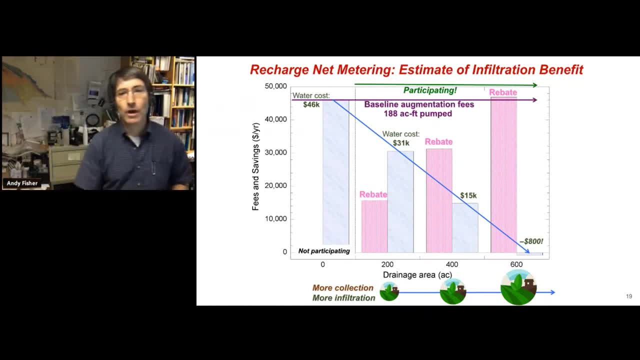 ground. So what does that mean in terms of water cost? Well, for the grower who doesn't participate, the cost is about $46,000 a year for water. For the grower with 200 acres of drainage, the cost is driven down by about 50 acres. 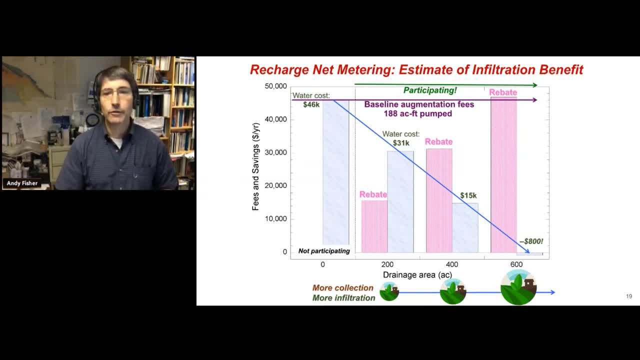 So that's a benefit. So the net pumping is reduced By about $15,000 per year And with a large enough drainage area, this grower pumps the full 188 acre feet, grows those delicious red berries and at the end of the year would get a check for $800. 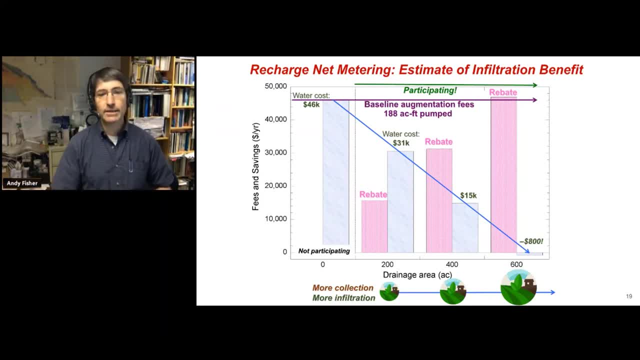 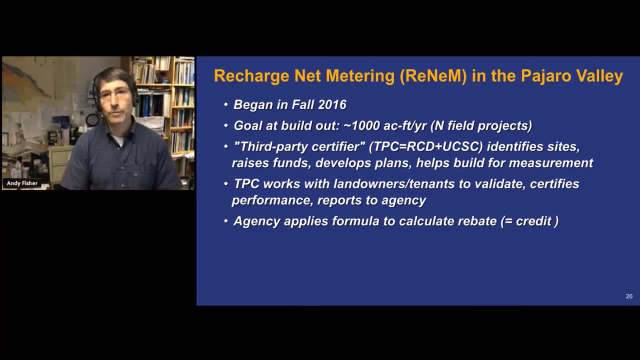 Because so much more water is being put in the ground than is being taken out. Well, this is more than a fantasy or a scenario. A group of us proposed to the board of directors for Pajaro Valley Water that they give us a try as a pilot project. And that's been running since the fall of 2016.. That is water year 17.. The concept is to get 1,000 acre feet- around 10% of the deficit- into the ground at build out. This is going to require multiple projects, not just one. 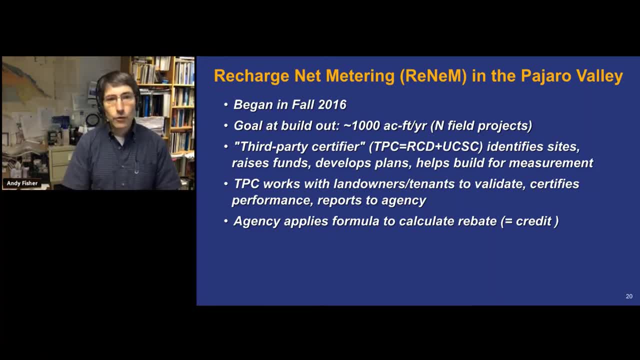 We at UC Santa Cruz, working in close collaboration with the Resource Conservation District of Santa Cruz County and, of course, with our stakeholders, we serve as the third party certifier, That is, we count the benefit, We deliver the benefit, We deliver a report. 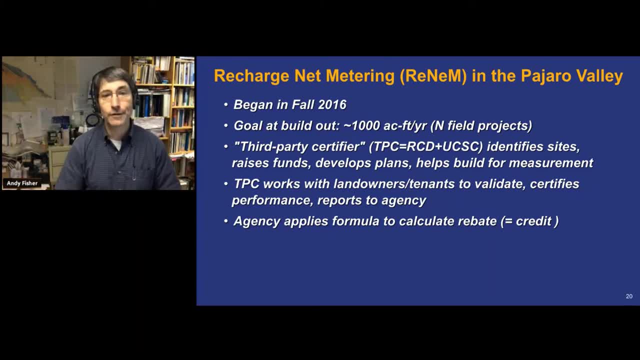 And everybody agrees in advance to accept our numbers and not argue with us about them. Then the agency helps by issuing the rebate on an annual basis. We work with landowners, We work with the agency to help identify sites. We want to build the projects so we can measure the benefit. 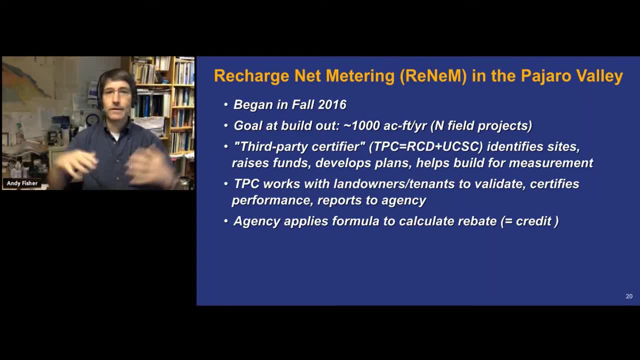 And that's important. If you have a whole lot of inflow coming from different places and you can't measure it, it's hard to quantify that benefit. So right now there are two active renum sites. That's Recharge Net Metering. 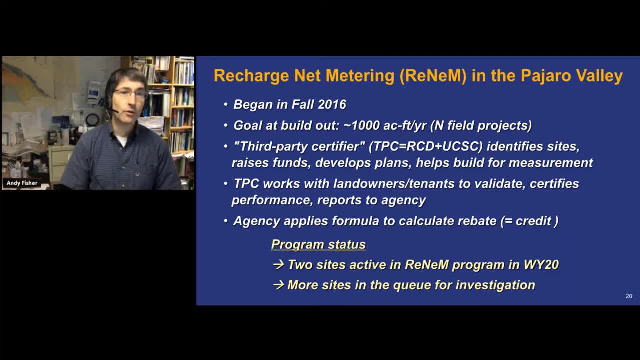 We have a lot of sites in the queue. One thing we weren't sure about was whether enough people would want to do this, that we could justify running a program. But frankly, at this point the biggest challenge is our own bandwidth, our ability to investigate. 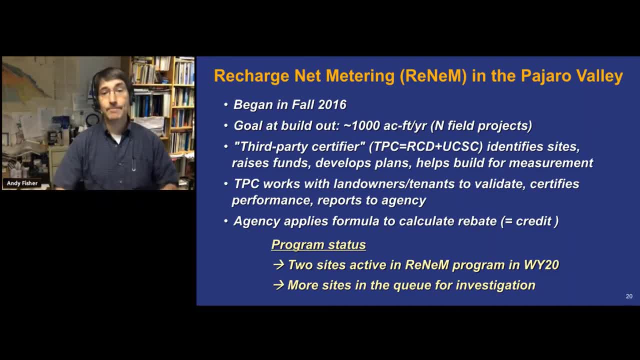 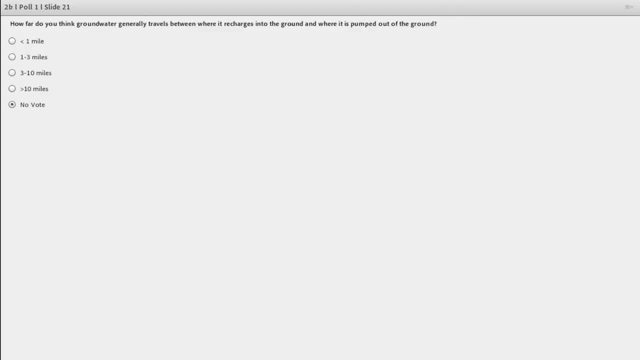 sites and evaluate and then get things set up in order to run projects. So that brings us to our first poll question. All right, Alex, I mean, Andy. How did our community react? How did our community react? How did our community react? 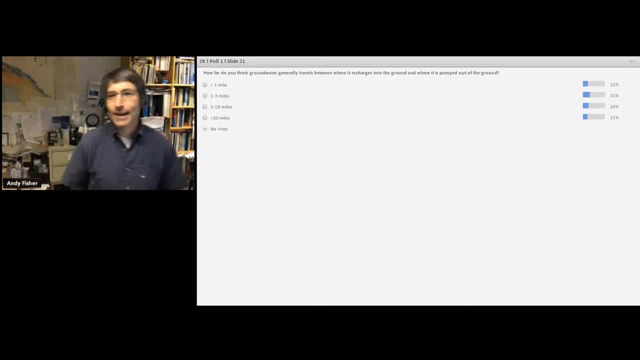 Yeah, Yeah, Everybody's a winner on this show. Of course, the answer really is all of the above, but you know, it really varies place by place and it probably varies year by year and it may even vary week by week. 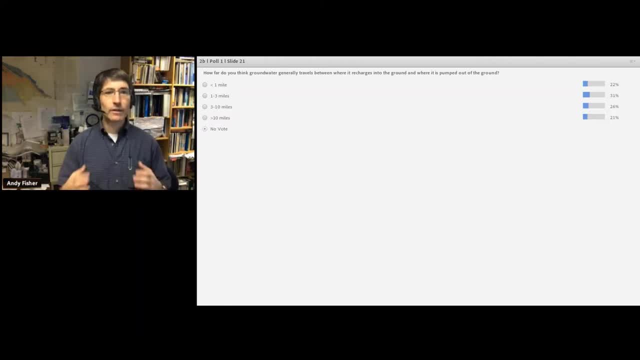 This is really a challenge in managing groundwater and it's one of the reasons when we think about managing water, we need to think about an entire basin, because different places are going to have different responses and they really are going to vary with time. 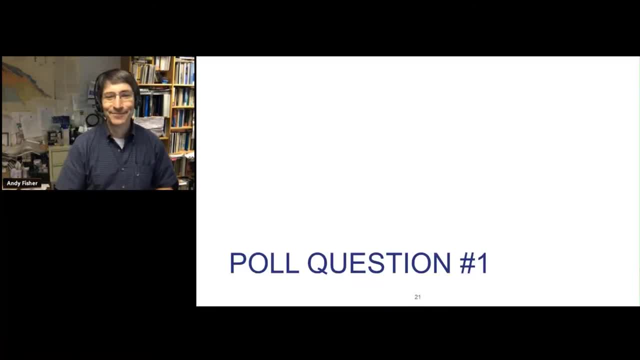 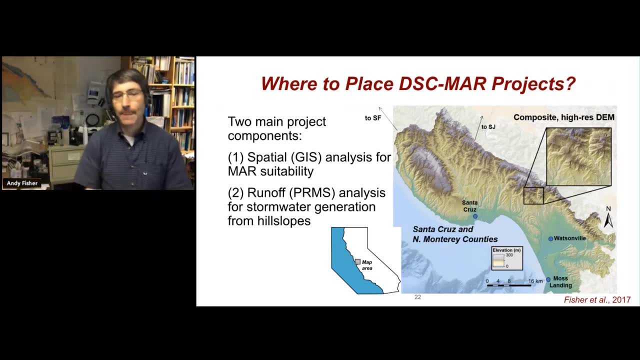 So let's go back to the talk, Thank you. So one of the challenges is to figure out where to put managed recharge projects, And we've done a couple of analyses in collaboration with regional water agencies. This map shows all of Santa Cruz. 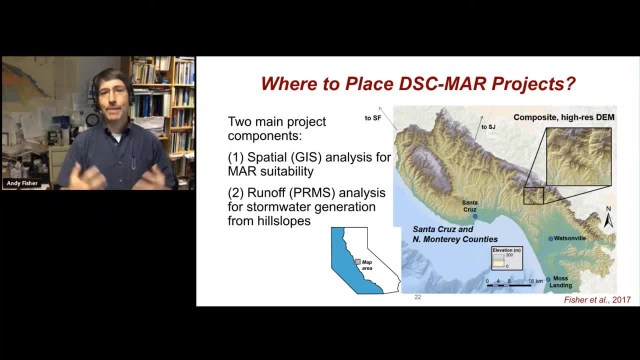 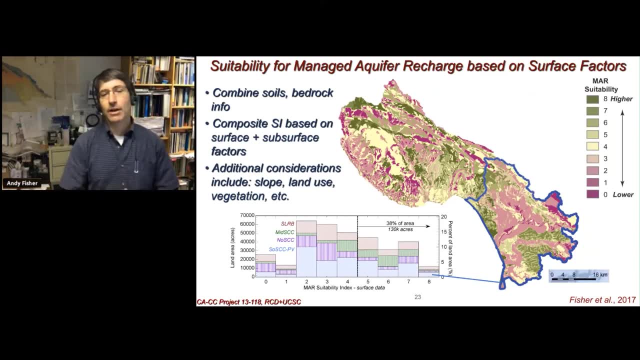 This map shows all of Santa Cruz County. We combined a bunch of datasets and did some modeling to try to figure out where groundwater might be improved through collaboration, Through collection of stormwater. So this is a suitability map we generated for recharge. The southern area here shows the Pajaro Valley. 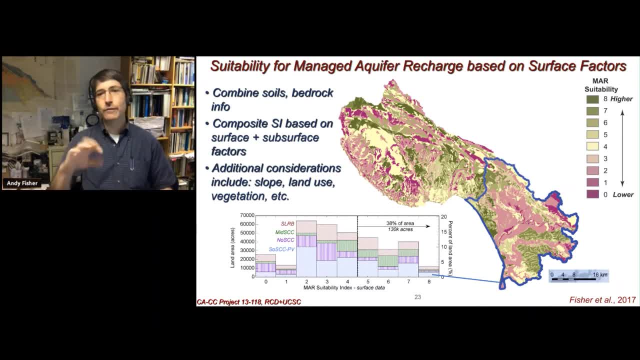 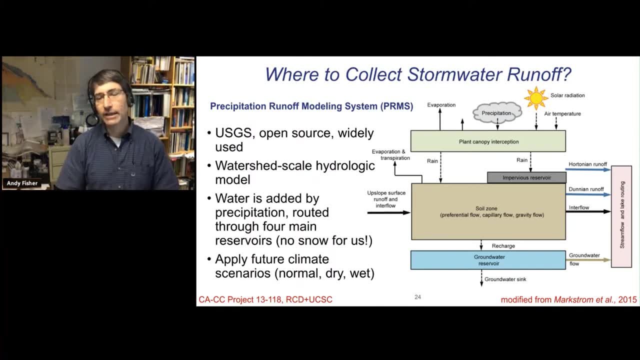 Areas in green are more suitable, And the key point here is these patches of green are scattered all over the valley, not just in any one place. We then took on a series of runoff modeling exercises to try to figure out how much water could actually be available. 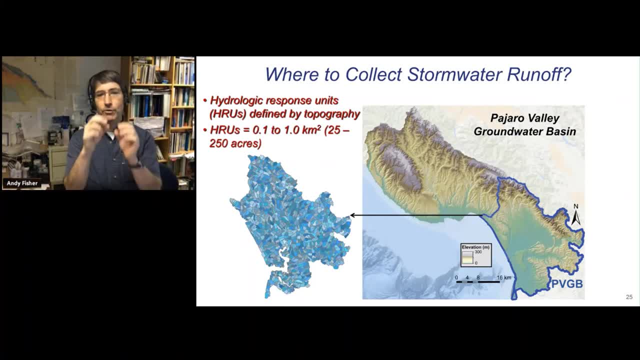 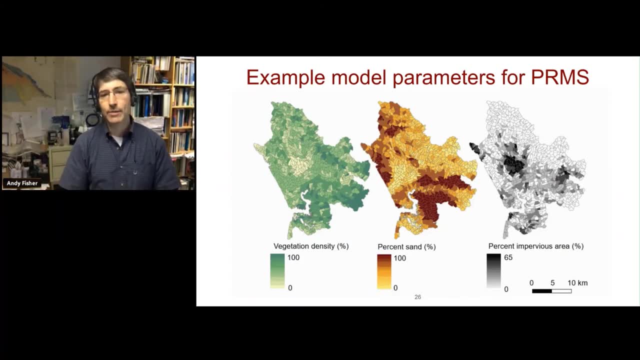 And to do this, we divided up the Pajaro Valley into a number of these little patches, Polygons, or hydrologic response units. In each unit, we assign more than 60 different parameters, Things like how much sand is in the soil. 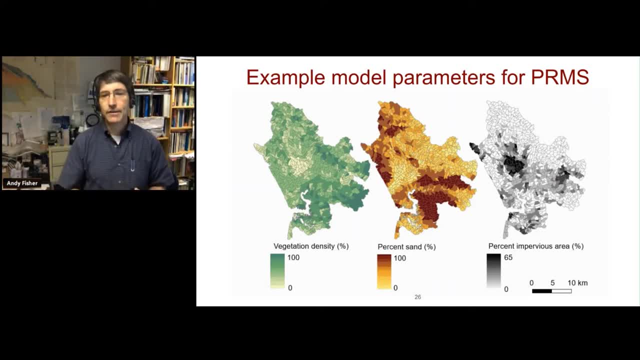 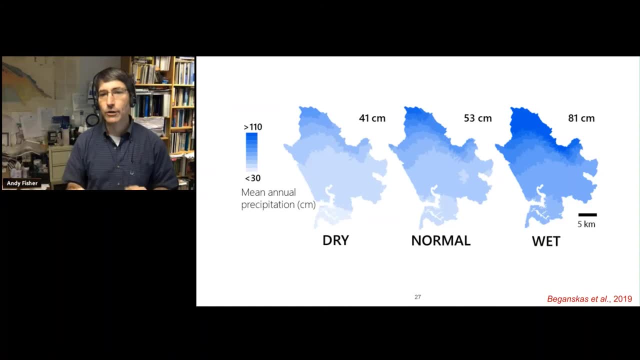 How much concrete makes the surfaces impervious, The density of vegetation, All kinds of data. And then we apply rainfall to the landscape. using historical, very detailed records from across the region, We create scenarios that are dry, normal or wet. 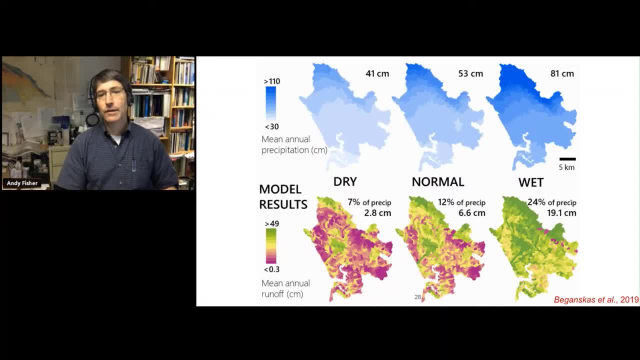 And here are some maps of runoff. So the pink is less runoff, Less runoff And the green is more runoff. And of course there are big differences. During wet years we get a lot more runoff. But you can also see how variable the runoff is. 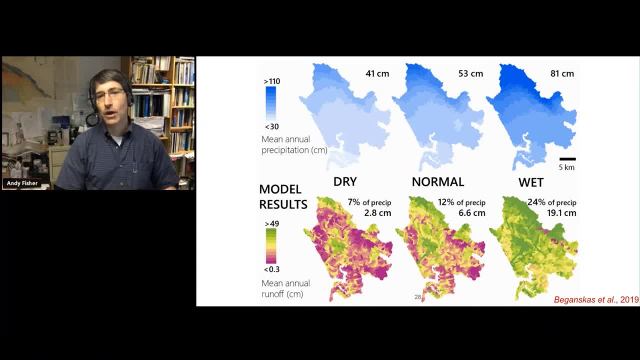 The city of Watsonville generates a lot of runoff because of all the concrete. These areas near the coast don't generate much runoff because of all the sand, So this lets us look in a very granular way at how much runoff is generated. We also looked at pre-development and contemporary land use. 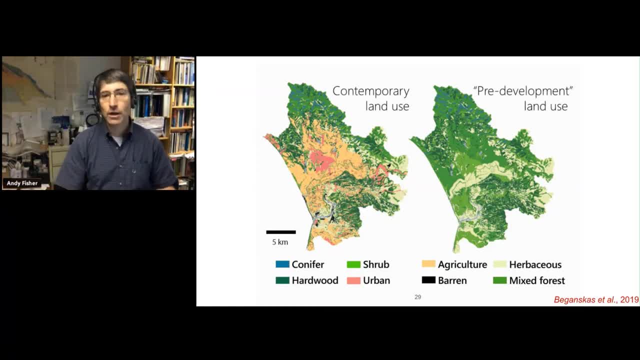 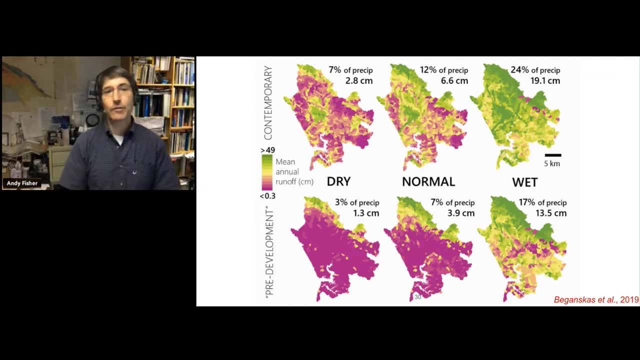 What's the effect of agricultural activity and urbanization on runoff generation. And this was pretty interesting. The lower map shows pre-development. All that pink means there was a lot more recharge and evapotranspiration before we developed the basin, And that's one of the reasons why the groundwater system is challenged. 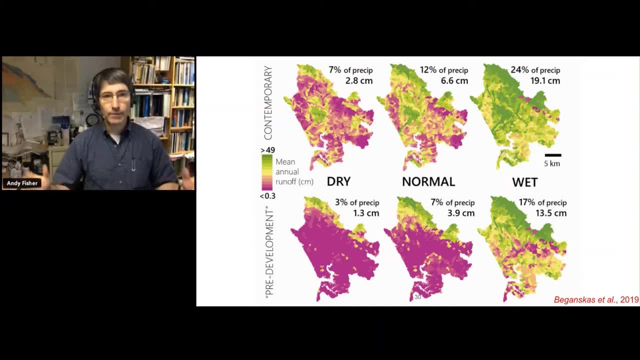 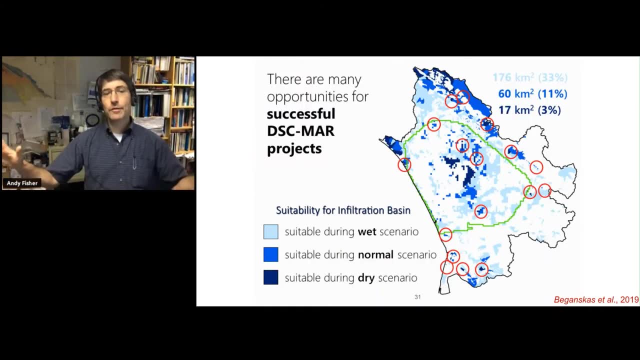 Because, frankly, there's less water going in over historical times, as well as more water being extracted. Now, one of the things we could do with these two sets of coverages Is put them together. We take our suitability map and we overlay it with our map of runoff generation. 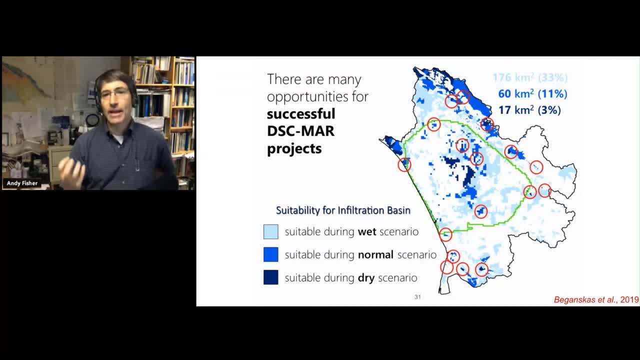 And the areas in dark blue. here are these patches of multiple acres where infiltration basins in principle could be placed if there was sufficient supply, And I just want to point out the site I showed you earlier on. Boca Risa Ranch is right here. 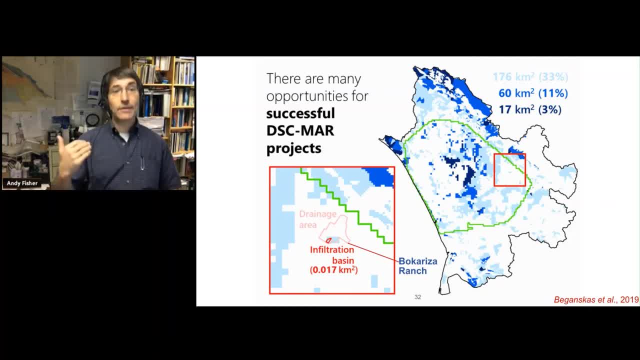 And that basin happens to be located over a little blue patch. that is highly suitable. In part it's because that's an ancient stream channel With coarse deposits that cuts across that part of the basin And by accessing that window we can get water into the ground. 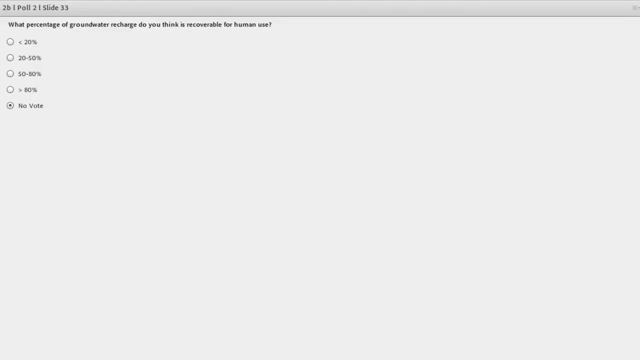 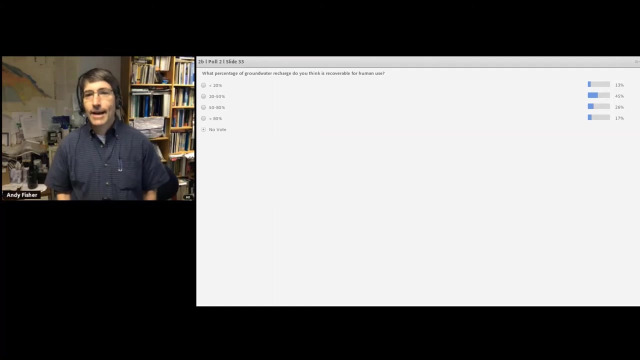 That brings us to poll question two: All right, pens down everybody, Andy. how did we do? Yeah, I think people are on the right track. My guess is, again: this is highly variable And it's again going to vary by place. 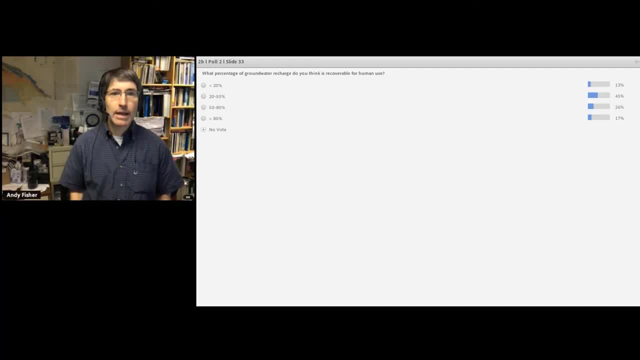 It's going to vary by time And even within a water year it can vary. So the numbers are going to be between 20 and 80 percent. You know, I've often said that a groundwater aquifer is a bank, like a colander is a bucket. 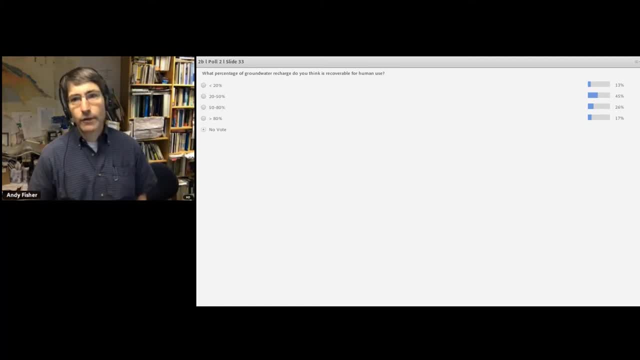 That water is on the move And there are rare cases where you can put water in and it sits there waiting for it to be pumped out, But in general that water is moving. Now you could think of that as loss at some level. 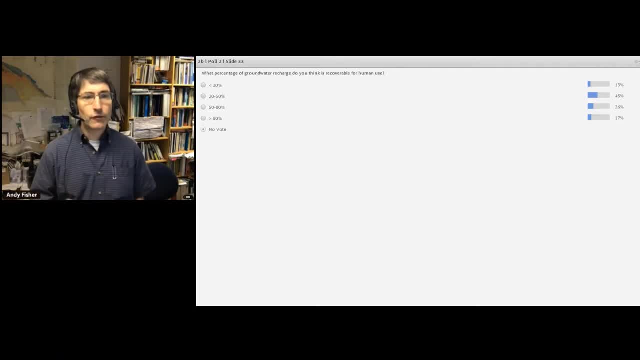 But it really is a benefit to many of the hydrologic system services that water on our landscapes provides. The movement of that water is flushing out solutes. It's providing base flow that supports streams. It's creating hard grounds along the coast that help to provide refugia and fish habitat. 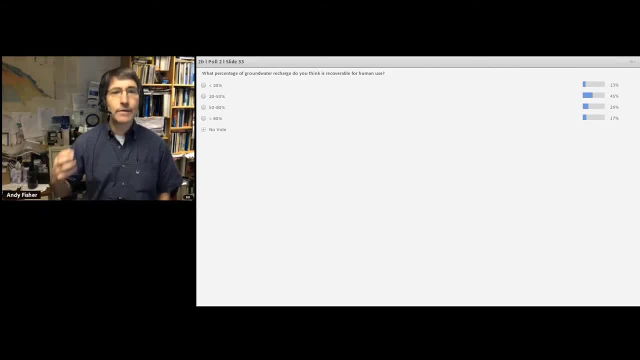 There's just a huge number of benefits that occur because of the movement of water. So if we think about groundwater recharge only in terms of storage, I think we're really missing a big part of the story, And I think the fact that it's not going to be 100 percent recoverable is fine as long 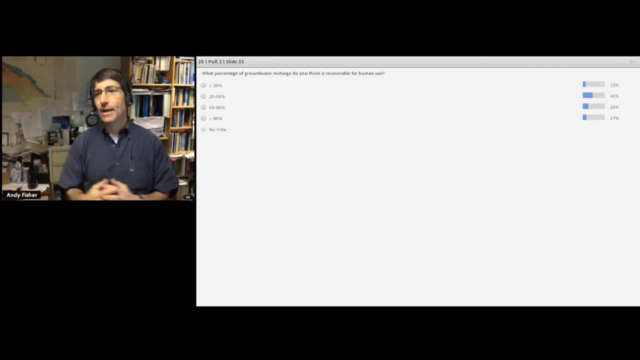 as we plan on that basis- And again, these are generalities that I'm talking about here- Individual projects certainly have higher amounts of recoverable water, So I'm going to wrap up the talk by telling you about a new project that we helped to. 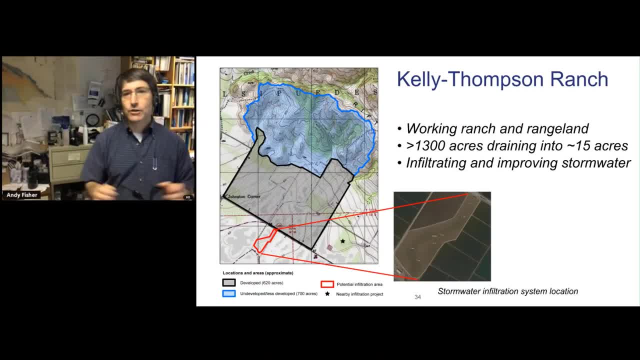 launch last year. that's very exciting. And this is at another ranch, Kelly Thompson Ranch. It's got a much larger drainage area supplying stormwater collection, In this case about 1,300 acres, The blue area that kind of looks like a little mushroom. 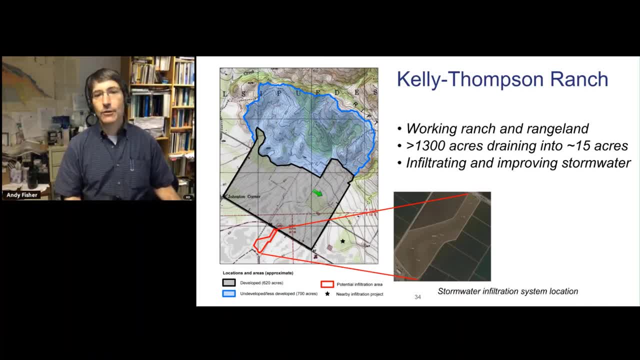 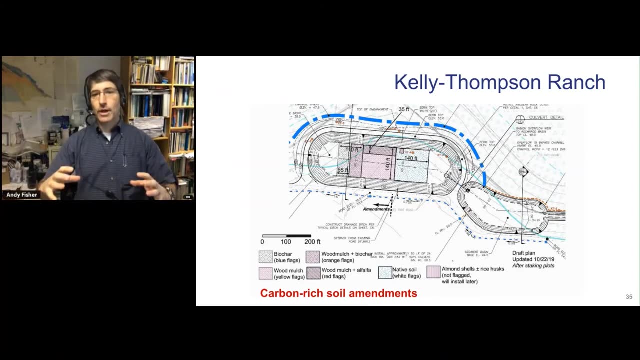 Over here. this is actually rangeland, and then there's irrigated cropland That drains into about a 15 acre parcel, a piece of which has been allocated for a recharge system, And this is an engineering drawing that shows the design for that system. 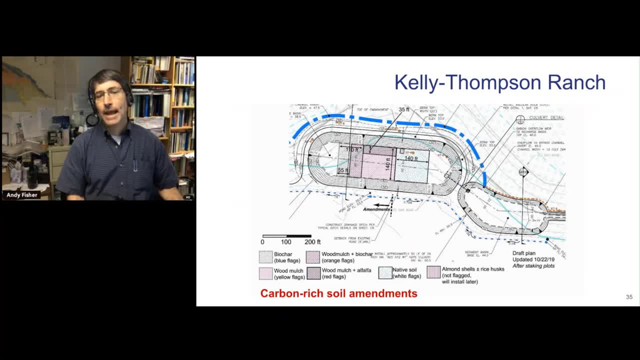 There's about a one acre sediment detention structure and then a gabion basket and a culvert that leads into a four acre infiltration basin And, in collaboration with our project, In collaboration with our RCD colleagues who were able to generate some additional support, 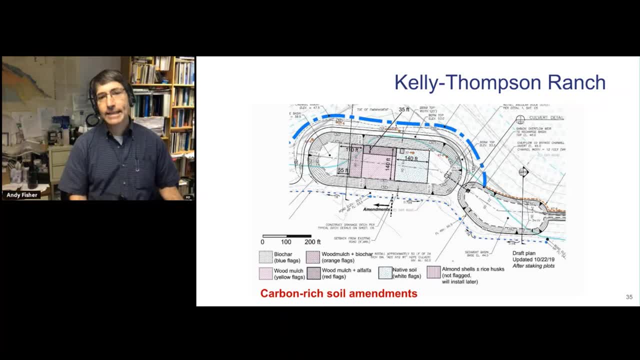 we were able, in the fall of 2019, to install a whole series of carbon amendments into the soil. One of the things that we've been working on is improving water quality during infiltration. I'm not going to have time to go into it during this talk, but I'm happy to answer questions. 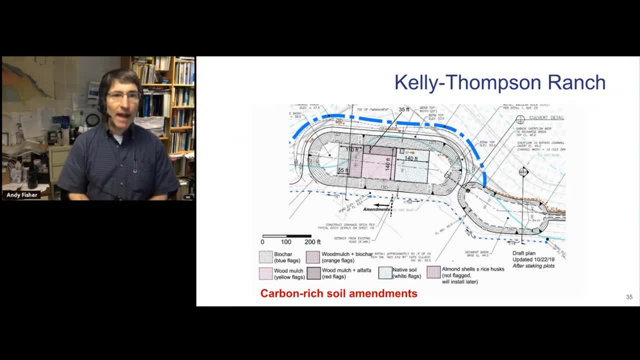 about it and direct you to some papers. but as water moves rapidly through the shallow soil And we're going to develop, if you have enough available bioavailable carbon, so that native microbes can help to consume nitrate and provide other water quality benefits, 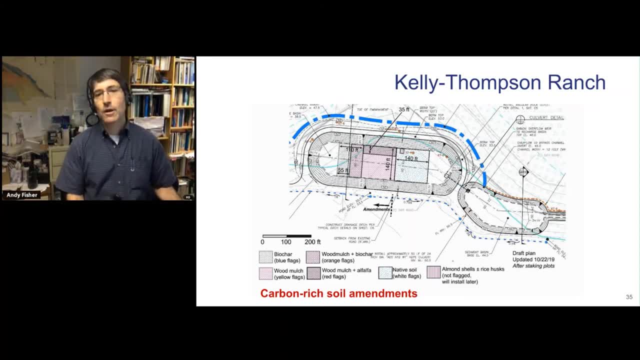 And we've been testing different materials: Biochar in this case, Biochar plus wood mulch, Wood mulch, Wood mulch with alfalfa And a patch with almond shells. This year we renewed that patch with almond shells and rice husks provided by a grower. 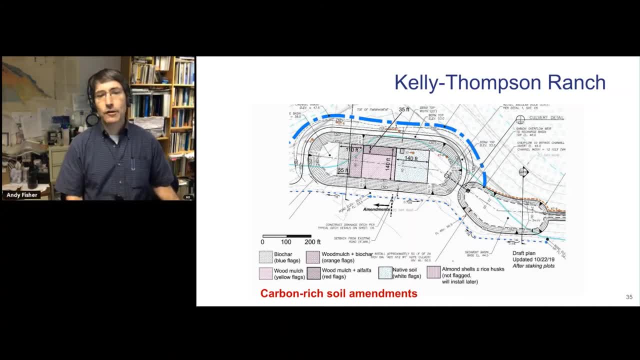 in the Central Valley And we have instruments in the system that we use to monitor that. So we've been testing different materials And we've been testing different materials monitor how it functions. So here's a panoramic photograph from last fall. 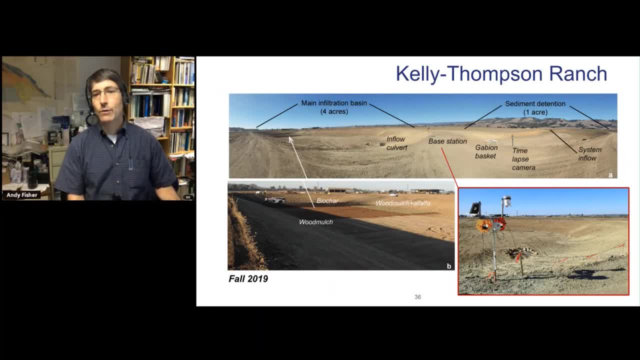 This is the sedimentation basin. These are the foothills to the right where the San Andreas Fault is located. Here's the gabion basket. a pipe leads into the main basin. here And the diagram the photo on the lower left shows. after all these amendments were blown. 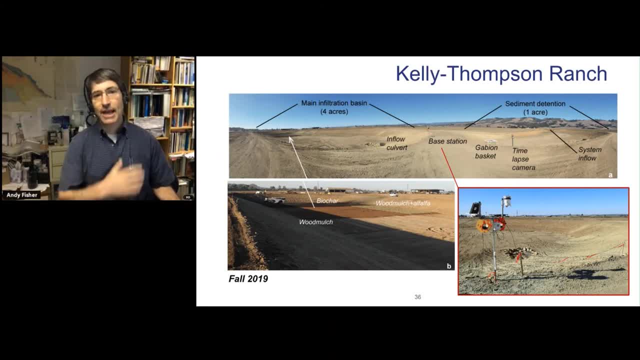 out into patches in the basin and then this giant tilling machine came across and then tilled them into the upper two feet of soil. We put out instrumentation- We just finished deploying these instruments for the current water year- and we're getting real time data returns so we can monitor the rainfall, the flow, the water level and then. 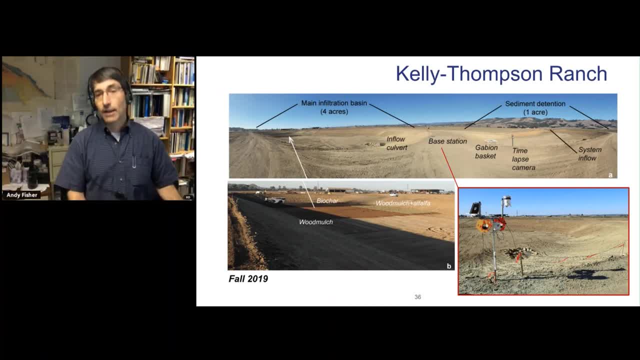 we can rush out and we can instrument or we can collect samples of fluid from the instruments we've already deployed. We have 18 locations monitored, with tubes coming up the side of the basin, where we're able to then pull water samples from in the basin and from below the carbon amendments. 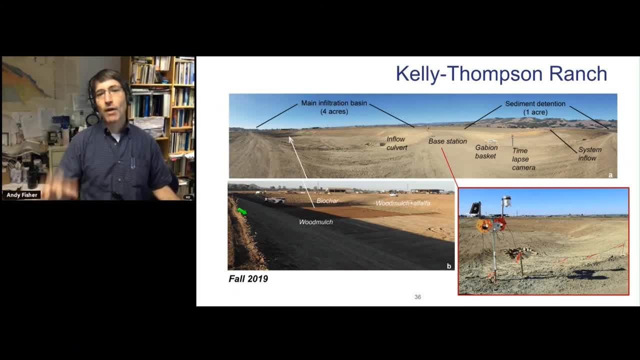 in order to document The improvements to water quality. We're processing data from last year. Things have been slowed down a bit because of COVID and our inability to get into the labs, but we're cranking through the samples and so far the results look really good with 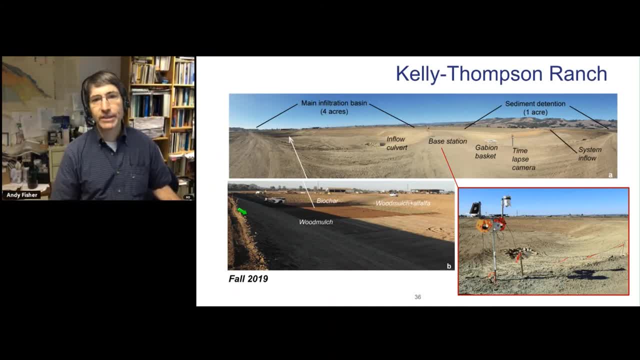 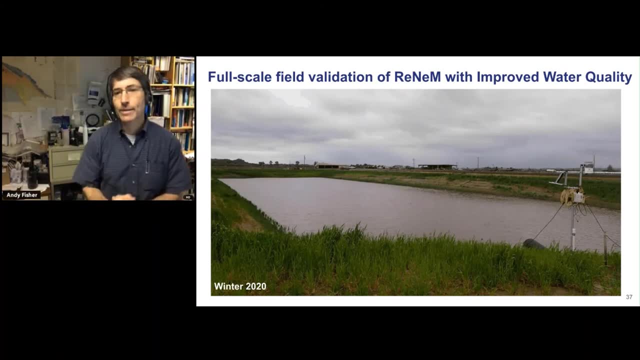 the wood mulch and the almond shells in particular, showing good results with nutrient load reduction. So this is that system operating last year when the basin was full, and here's our real time instrument sending us data back. Last year we certified for this project about 100 acre feet of infiltration benefit and 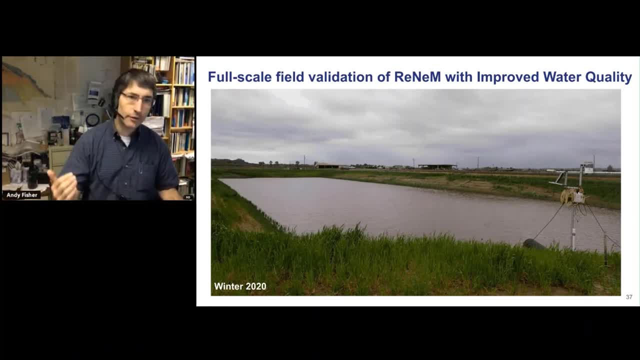 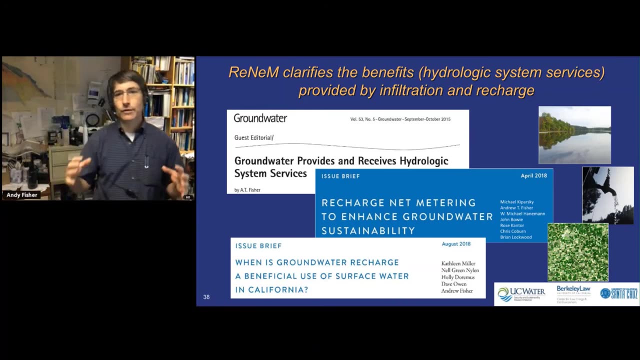 that generates a rebate then for that landowner, but we're also demonstrating a net improvement to water quality relative to the local ambient groundwater. That's very important for not just not degrading the groundwater but for actually improving the groundwater. So all of this really serves to summarize that groundwater recharge is itself providing 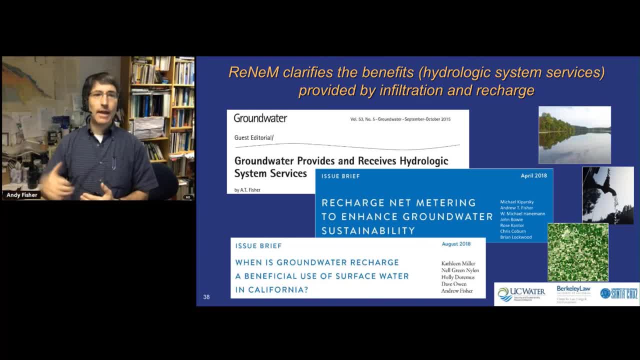 a variety of benefits. I'm not claiming that recharge equals beneficial use, but I'm claiming and we can show that recharge generates many benefits to individual users but also to the basin as a whole. And the recharge net metering program, I think, is important, in part because it really helps. 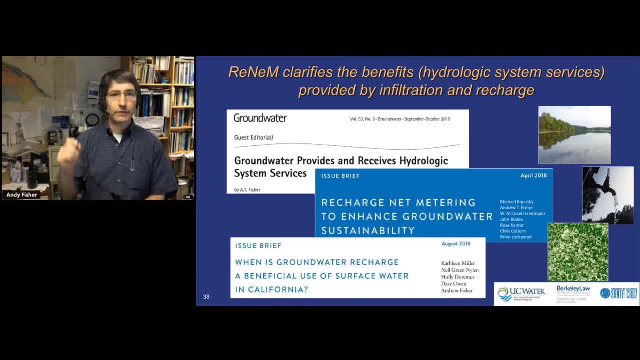 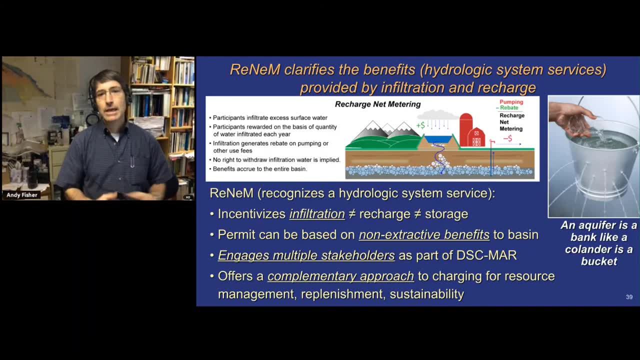 to give us a good justification for quantifying those benefits, for making the measurements, collecting the samples and demonstrating that improvement. Thank you, Recharge. net metering is different from other kinds of incentive programs, but it does share characteristics with other programs. One of the characteristics that's unique is that we incentivize infiltration rather than 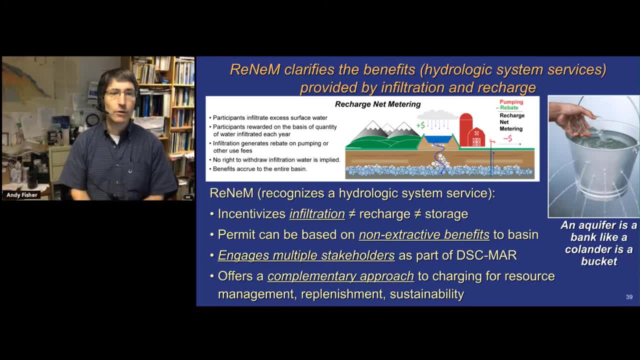 recharge, because infiltration is relatively easy to quantify and measure and it does generate benefits. Also, we're able to engage a lot of different stakeholders around the basin and distribute benefits around the basin. It's not an approach that's going to be applicable everywhere and even in other basins. 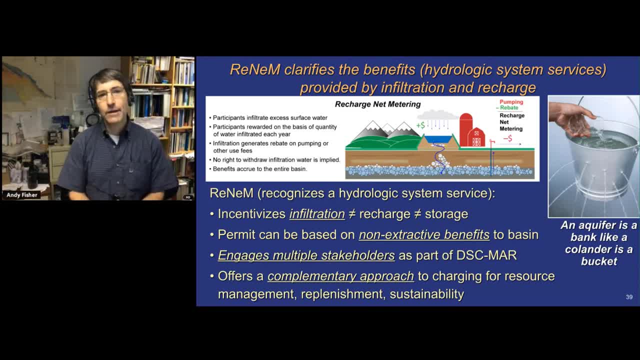 where it can be applied. it may need to be modified, But I think this idea of recognizing the benefits of recharge and providing incentives based on measurable benefits has value, certainly in the Pajaro Valley, but I think potentially in other basins around the state, and that's something else that we're also working on.